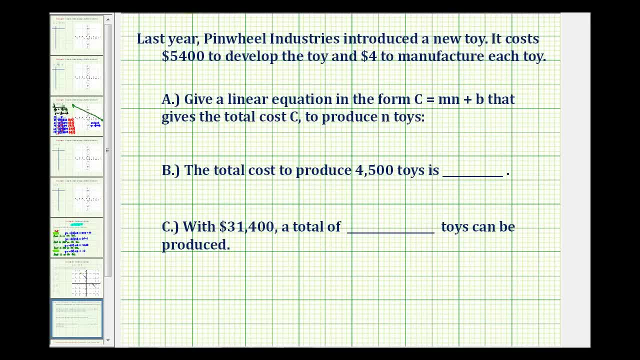 Here's an example of an application problem that can be solved using a linear equation. Last year Pinwheel Industries produced a new toy. It cost $5,400 to develop the toy and $4 to manufacture each toy. We want to give a linear equation in the form of: C equals M times N plus B. 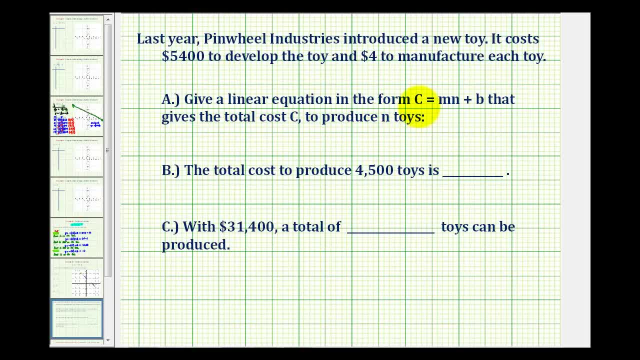 that gives a total cost C to produce N toys. So our equation is going to contain the variables C and N, which means we need to determine the value of M and the value of B. Notice that M is being multiplied by N, which is the number of toys produced, and B is a constant. 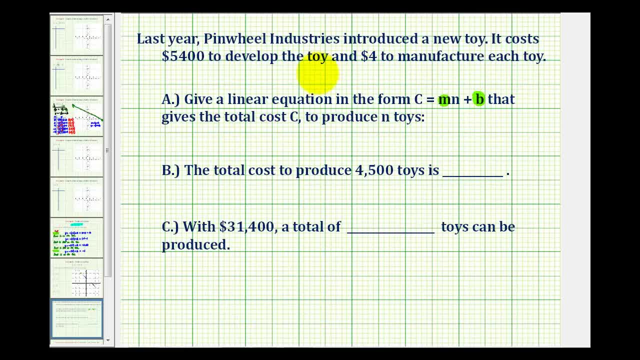 So, looking at the information that we're given, it costs $5,400 to develop the toy. so this is going to be the cost, regardless of how many items that we produce. But then there's an extra cost or the manufacturing cost of $4 for each toy. 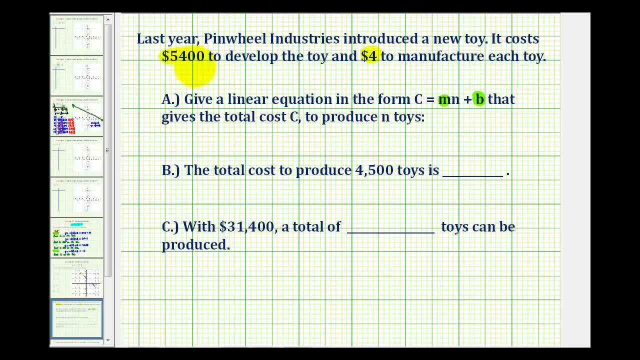 So if we produce zero toys, it's going to still cost us $5,400.. If we produce one toy, it's going to be $5,400 plus 1 times 4.. If they produce two toys, it's going to be $5,400 plus 2 times 4, and so on. 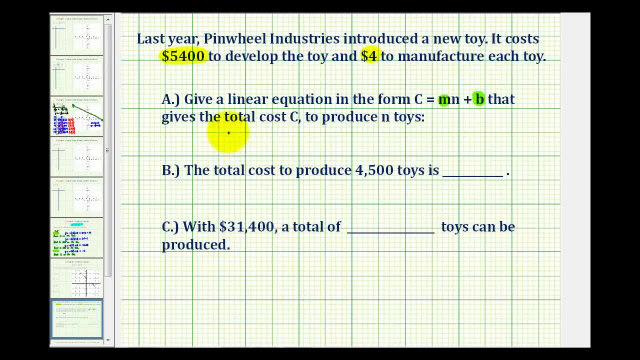 So with this information we can write the cost equation where C is going to be equal to $4 times the number of toys produced, so 4N plus the fixed cost, which would be $5,400.. Normally, in the end we're going to have $5,400. 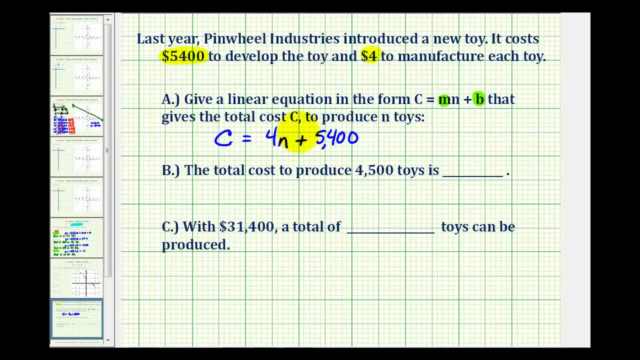 In the equation the units are left off with the description of what the variables represent. For Part B, we want to know the total cost to produce 4,500 toys, where in this case 4,500 would be N- the number of toys produced. 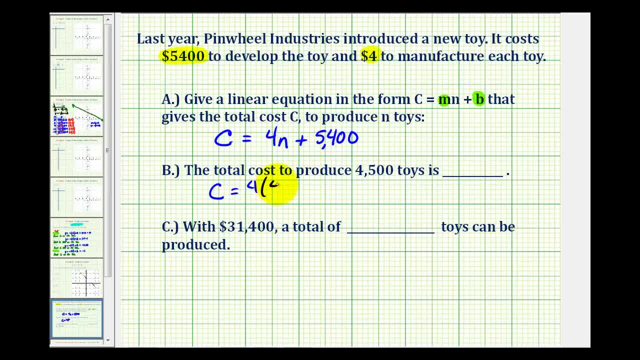 So we would have C equals 4 times 4,500 plus 5,400.. Well, 4 times 4,500 is 18,000, plus 5,500.. So we have C equals 4 times 4,500 plus 5,400. So we have C equals 4 times 4,500.. So we have C equals 4 times 4,500 plus 5,400.. So we have C equals 4 times 4,500 plus 5,400.. So we have C equals 4 times 4,500 plus 5,400..